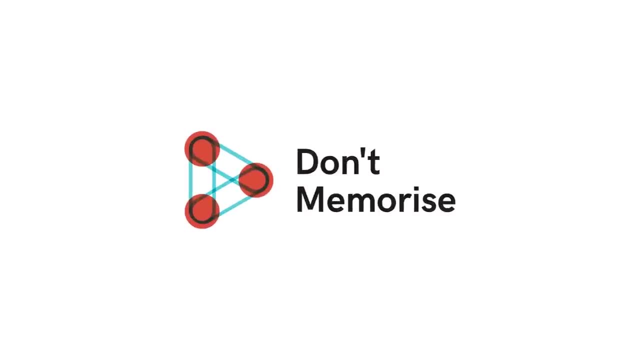 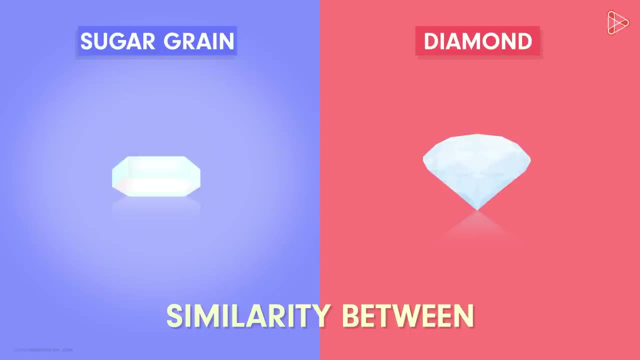 If I ask you what is the similarity between a sugar grain and a diamond, maybe you'll say that they both are lustrous. And what if I ask you the similarity between a diamond and a graphite? A graphite is just this piece of black stone used in laboratories. Maybe. 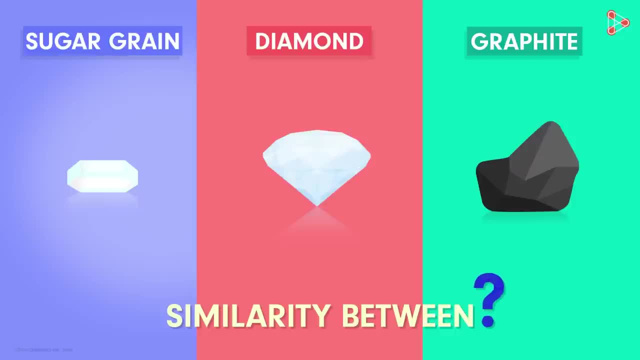 you'll think there is no similarity. Is there really no similarity between these two? The answer would surprise you. There is something common between all these three things. I'm referring to the element that these three are made up of. I'm referring to carbon. 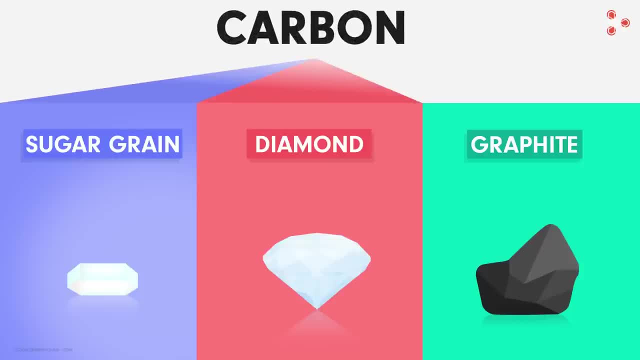 Wait a second. Are we saying that the sugar, the radiant, diamond and graphite are all made up of carbon? Absolutely? In fact, diamond and graphite are almost pure forms of carbon. They are majorly made up of carbon, with a few minuscule elements that come as impurities. 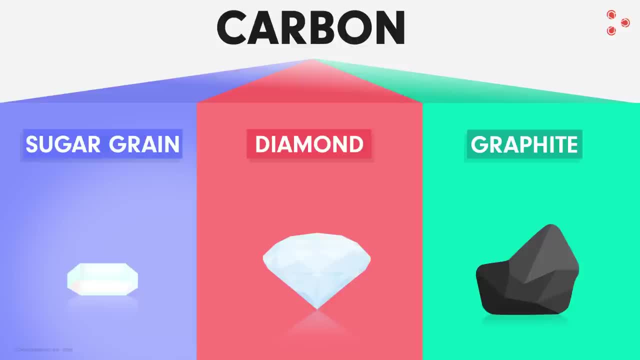 But how can there be so much difference in the looks of different materials made up of the same element? How can it be possible that the substances made up of the same element- carbon- appear totally different? And wait, they also have different chemical properties. The looks are different, the chemical properties are different, but they are made up of the same. 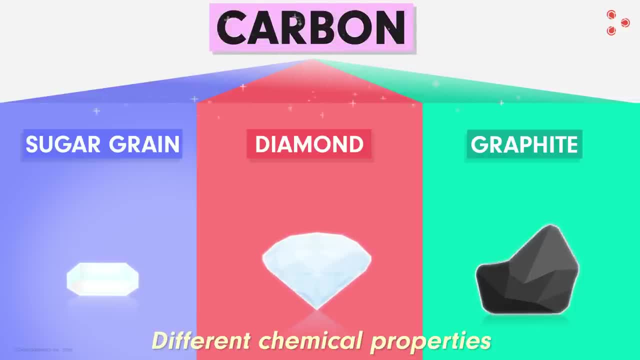 element carbon. Is this some kind of magic? Well, the magic lies in the element itself. The element carbon has several interesting properties, And that's what makes it special. It is capable of forming bonds with most of the elements. That is the reason why carbon. 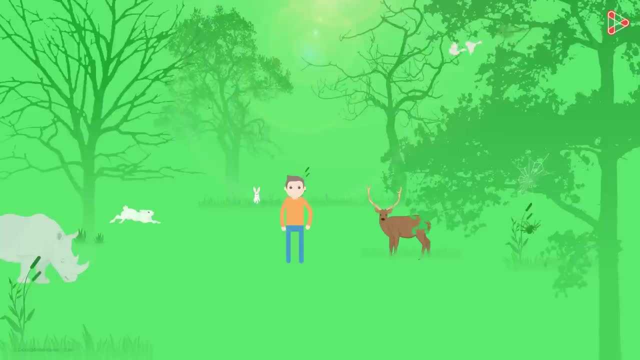 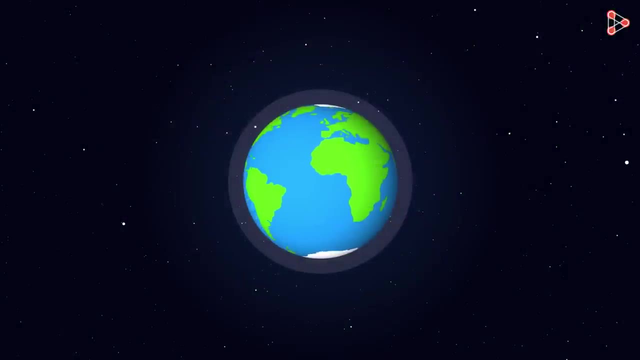 compounds are quite commonly found everywhere, But did you know that carbon is actually present in very small quantities in the earth's crust and also in the atmosphere? That's the irony: In spite of being present in almost every compound around us, carbon accounts for almost less than 1% in the atmosphere. That's the irony. In spite of being present in almost every compound around us, carbon accounts for almost less than 1% in the atmosphere. That's the irony, In spite of being present in almost every compound around us: carbon. 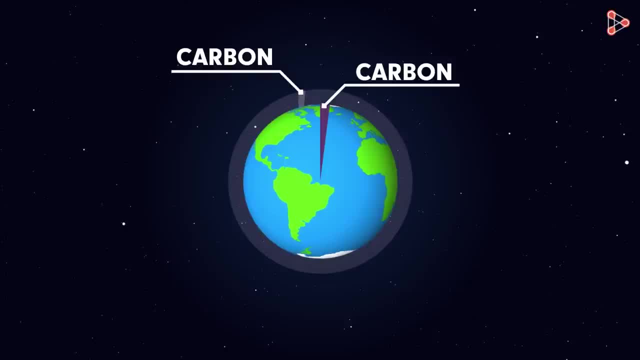 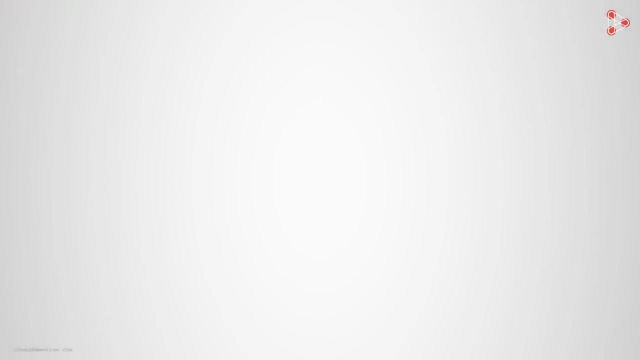 accounts for almost less than 1% in the atmosphere. But have you ever wondered what makes carbon so unique? What gives carbon the capability to have so many different properties? Let me give you a hint. Can you tell me what are the chemical properties of elements based on? Yes, they are mainly based on the atomic